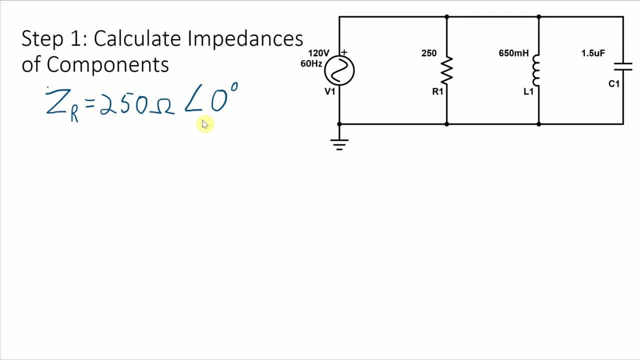 the impedance of the resistor And since it's a resistor, the phase angle is zero degrees. The impedance of the inductor is frequency dependent. It's equal to 2 pi times the frequency, which is 60 hertz times the inductance, which is 0.65 henries. This calculation will give me the reactance. 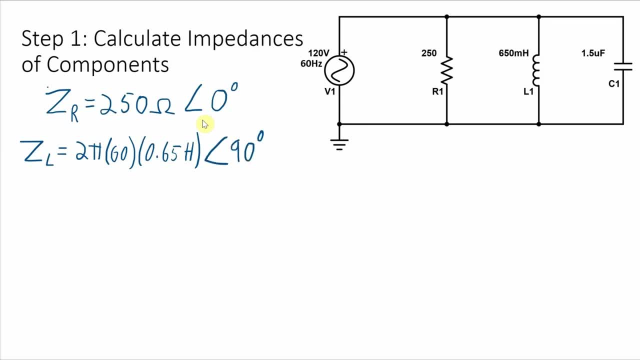 And then the phase angle is 90 degrees because it's an inductor. When I plug those numbers into a calculator, I get 245.04 ohms With that phase angle of 90 degrees. And then finally the calculation for the impedance of the. 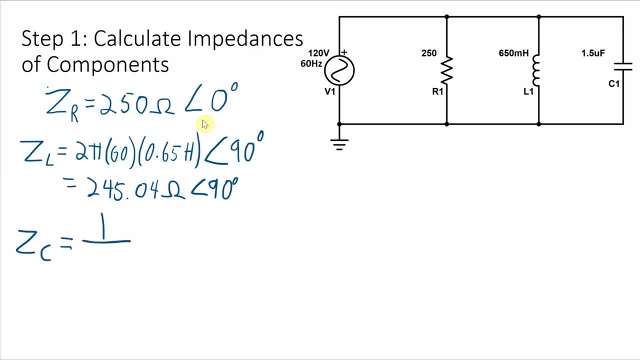 capacitor. Well, that one is also frequency dependent. It's 1 over 2 pi times the frequency times. the capacitance of 1.5 microfarads Gives me the magnitude, and the phase angle for capacitance is minus 90 degrees. When I plug those numbers into a calculator I get 1768.4 ohms And again that phase angle of 90 degrees. 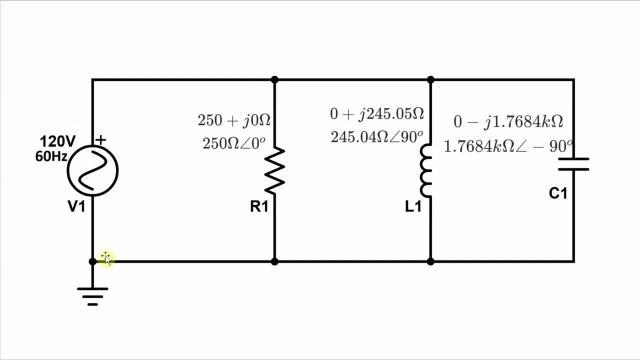 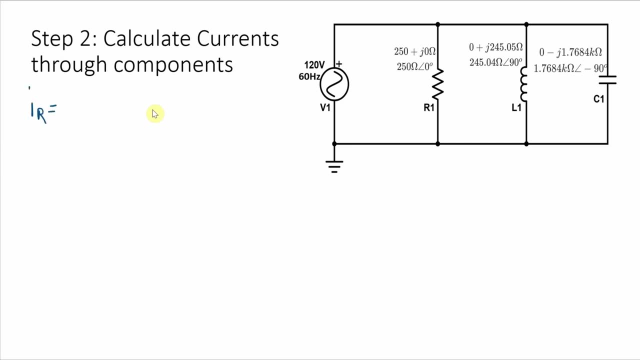 So I can put those numbers on the schematic. and I've put them on in both rectangular notation as well as polar notation. Okay, now I'm going to calculate the currents through each one of these components. Let's start with the resistor. The current through the resistor is the voltage across it divided by its impedance. 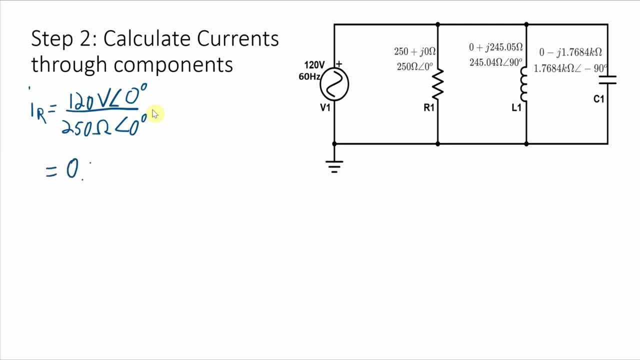 To do this calculation, I divide the magnitudes to get 0.48 amps And I add the phases to get 0.48 ohms. To do this calculation, I divide the magnitudes to get 0.48 ohms And I add the phases to get 0.48 ohms And I add the phases to get 0.48 ohms. 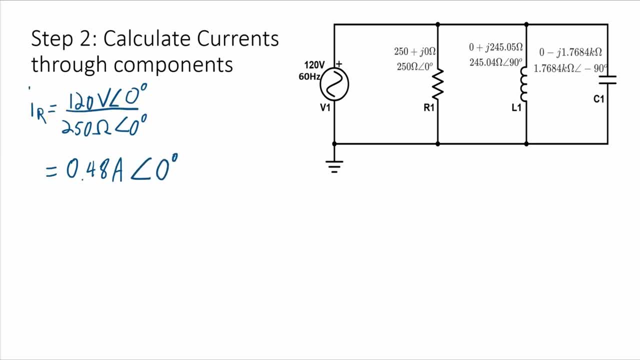 To do this calculation, I divide the magnitudes to get 0.48 ohms And I add the phases to get 0.48 ohms And I add the phases to get 0.48 ohms And of course I can convert this into rectangular notation. 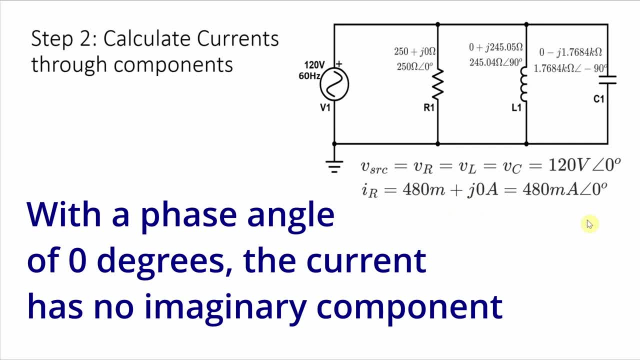 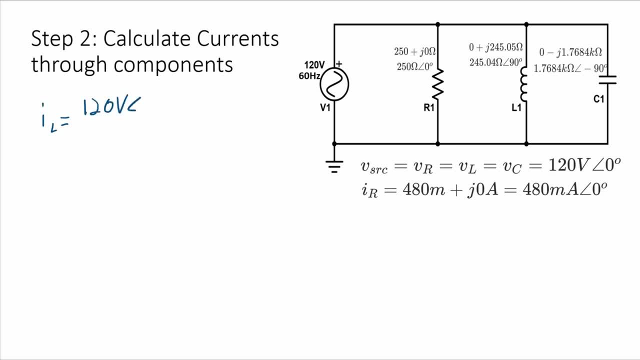 And I've got the values here in both rectangular notation and polar notation. Next current to calculate is the current through the inductor, Again voltage across the inductor divided by its impedance. Divide the magnitudes and subtract the denominator phase from the numerator phase, So I get 0 minus 90 for a phase angle of minus 90 degrees. 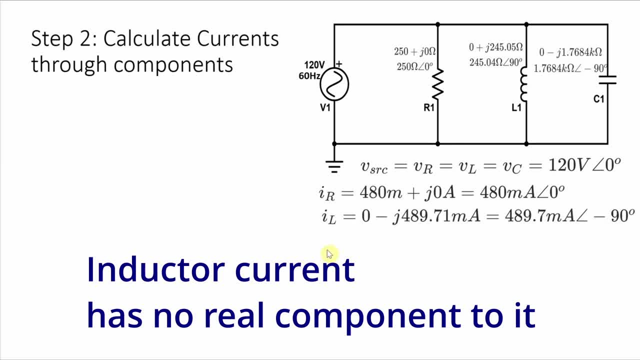 I can also convert that into rectangular coordinates And I've got that written out right here: 0 minus j, 489.71 milliamps or 489.7 milliamps, with a phase angle of minus 90 degrees. Last individual current to calculate is that through the capacitor. 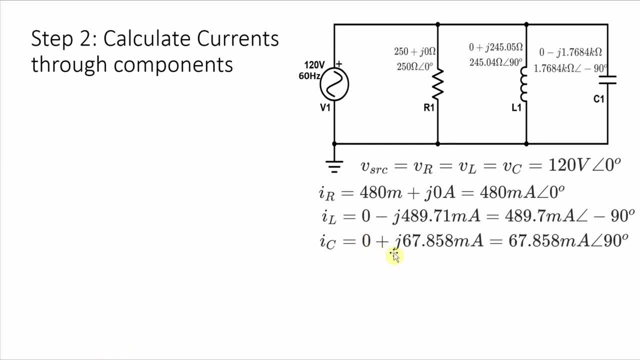 And when I convert that into the rectangular coordinates I get 0 plus j, 67.858 milliamps or 67.858 milliamps with a phase angle of 90 degrees. To calculate the total current or the current that's coming from the source, I can use Kirchhoff's. 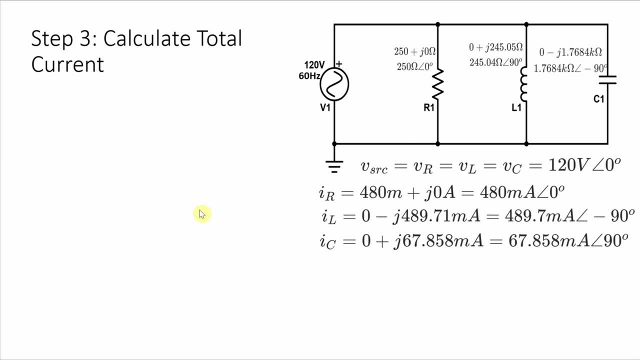 current law and see that the current coming from the source gets split through the resistor, the inductor and the capacitor. So the total current is equal to the current through the resistor plus the current through the inductor plus the current through the capacitor. 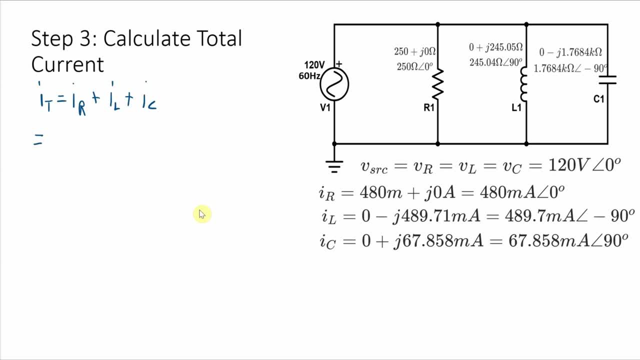 To do this addition I can take the values as they are in rectangular coordinates, Add the real parts together. I get 480 milliamps plus 0 plus 0. So that's 0.48 amps. And then add the imaginary parts, So I've got 0.48 ohms. And then add the imaginary parts, So I've 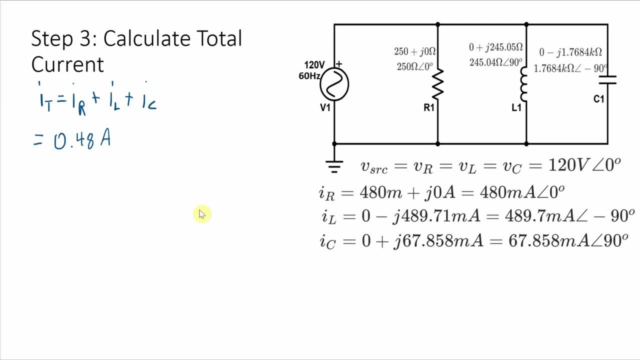 So I've got 0 minus 489.71 milliamps plus 67.858 milliamps, So that gives me minus j, 0.4218 amps, And in polar coordinates that's equal to the square root of 0.48 squared plus 0.4218 squared for the magnitude. 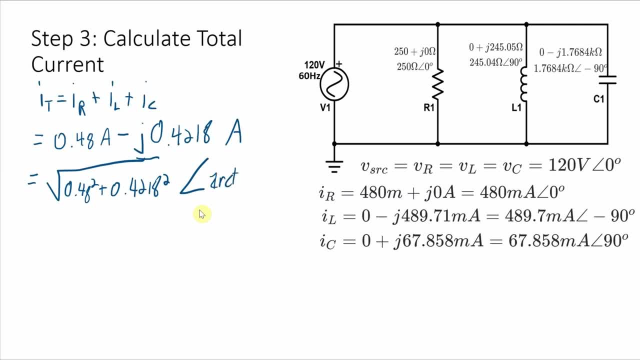 And the phase angle will be the arc tan of negative 0.4218 divided by 0.48.. Plug those numbers into a calculator and I get 0.639 amps. phase angle of negative 41.31 degrees. And there's my values for my currents all over here on the right hand side underneath the schematic. 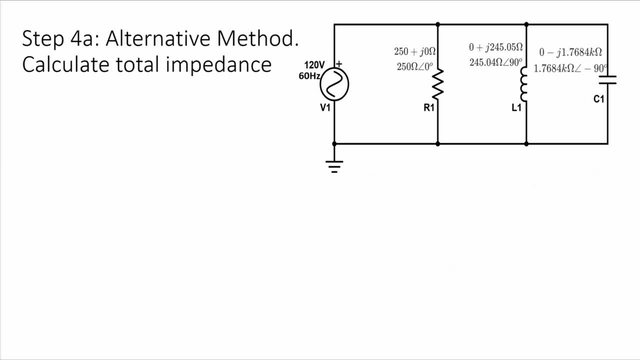 Now let's look at an alternative method to figure out what that total current is, And that involves first calculating the total impedance. So total impedance, because these impedances are in parallel, is equal to the sum of the inverses of the individual impedances to the negative 1.. 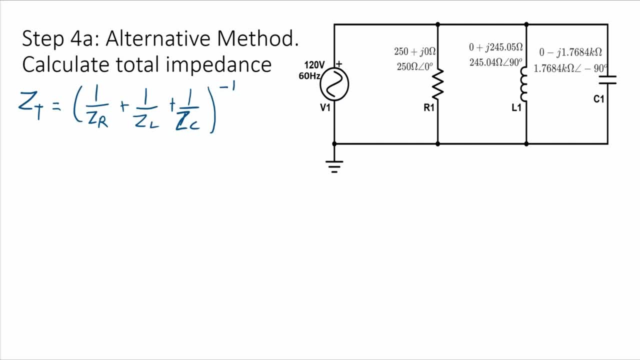 So in other words, it's the inverse of the sum, of the inverses of the impedances. So if I plug those values in, I get, And then I do each one of these inverses And then I need to add these together. 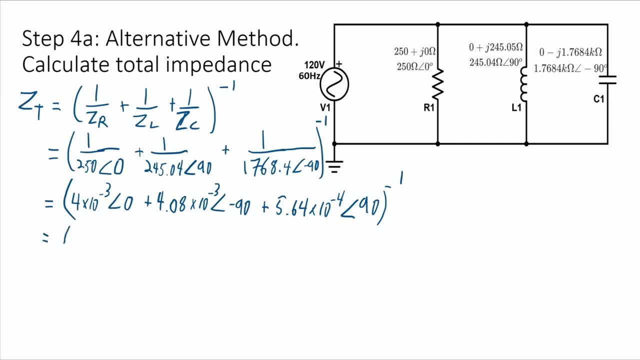 And it's probably easiest if these are in rectangular coordinates. So add the real parts- I only have this- 4 times 10- to the minus 3. And add the imaginary parts Now to get the inverse of this. I want this value in polar coordinates.